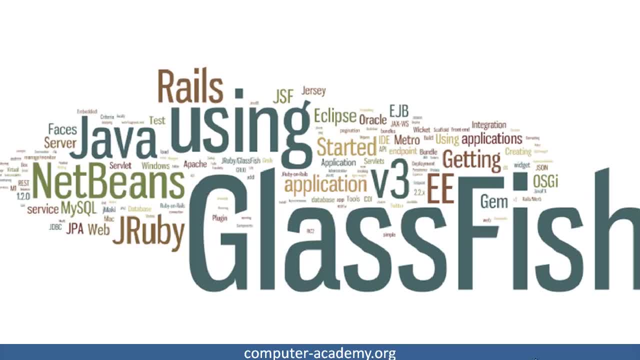 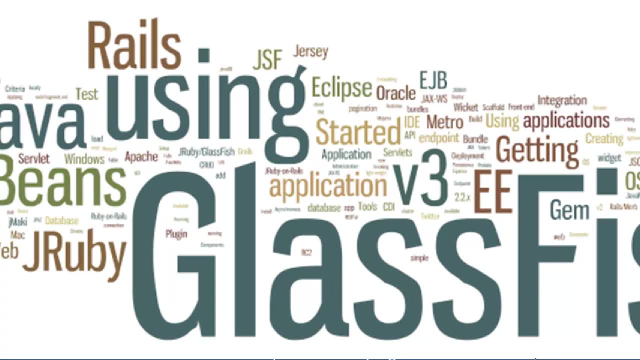 in the automotive industry. I hope you enjoyed it. Remember, if you want to learn more about the industry, in the next few videos I'll give you an idea of how you can work and have some fun with it, And we will also have some dates as an additional bonus where you can get a download and an 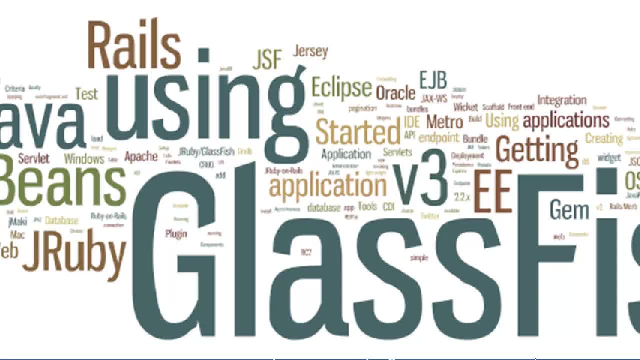 overview of the questions that you may have received during the session apologized affairs of your office that you can discuss in the next few days. Thanks for watching. I hope you enjoyed this. If you liked this video, how about always leaving your comments below? 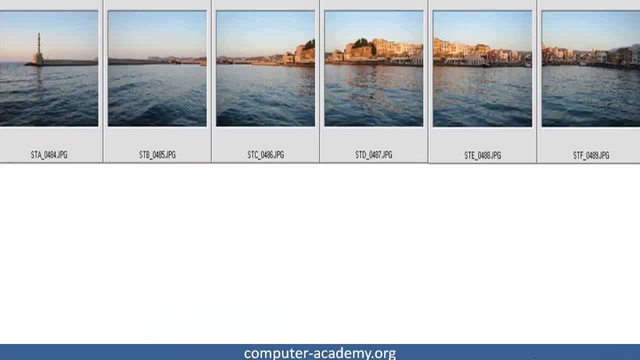 And you can also follow me on social media with my account, Facebook and Twitter, by clicking on the little icon on the right right corner. And remember, all I want to say is that I'd like to thank you very much for your support for doing this video. 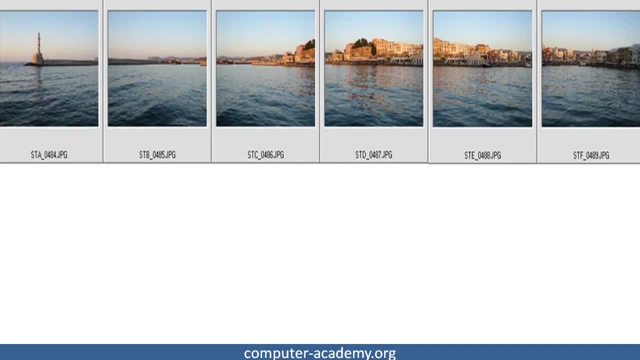 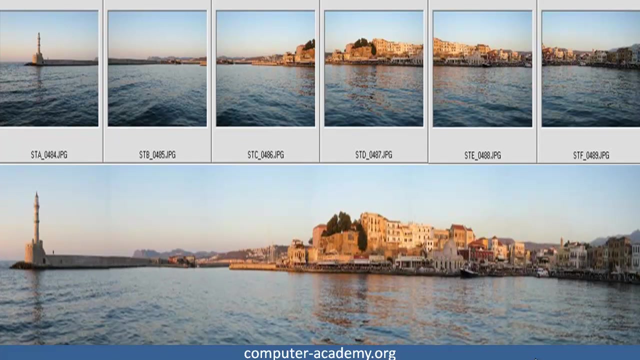 Let's break down the whole subject into small bits and study each area through simple explanations and then put it all together so you can see the big picture. The format of these videos has been inspired by some wonderful work done by the Khan Academy, and I hope you get a few minutes to visit it. 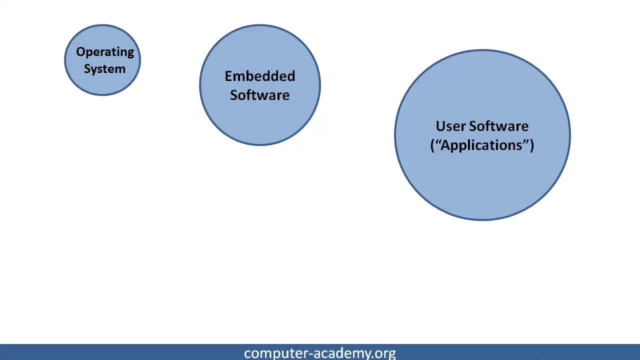 Let's start by looking at the types of things that computer programmers make. There are many, but broadly they can be categorized into three main buckets: Operating systems: the smallest bubble employs the fewest number of people in the industry. Examples include things like Windows 7, Mac, which help run your computers and laptops. 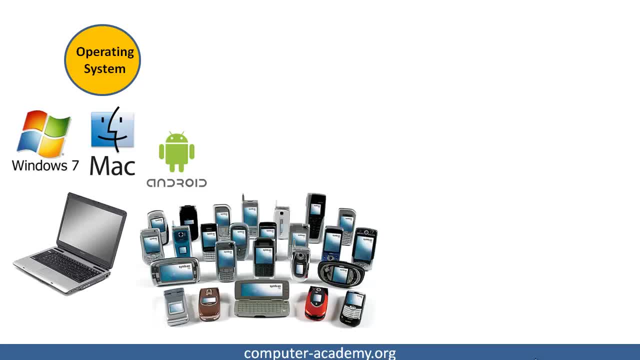 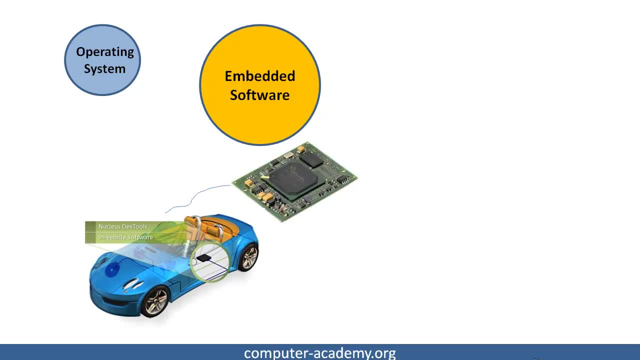 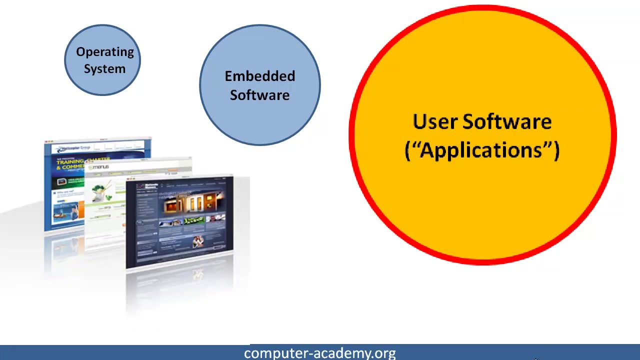 and software like Android that run your smartphones and tablets. Embedded software are things that run inside machines such as cars to control the engine. They help planes to fly and land safely and keep food cold in your refrigerator. User software is the largest bubble and represents things like websites, business applications. 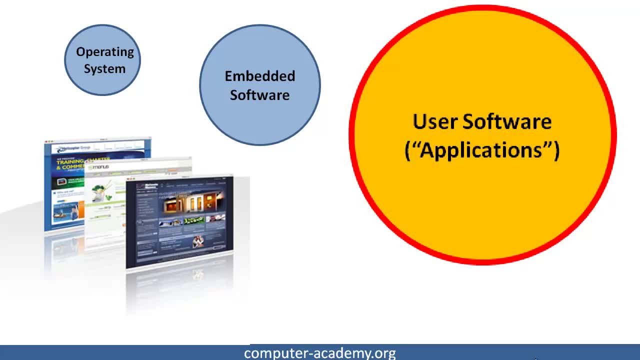 such as those used by your phone company to calculate your monthly phone bill. personal applications such as listening to music, typing documents, creating spreadsheets- Let's call this whole group applications. We will focus on this category of software, as it is the one that employs the greatest. 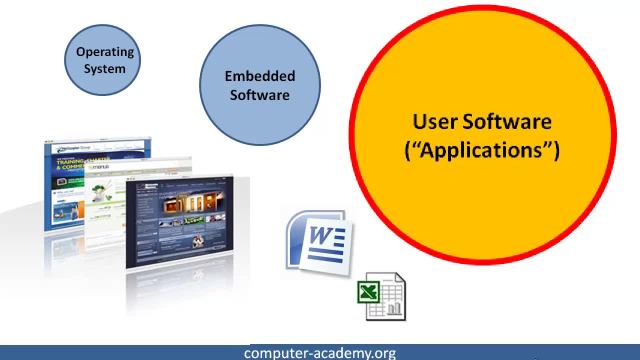 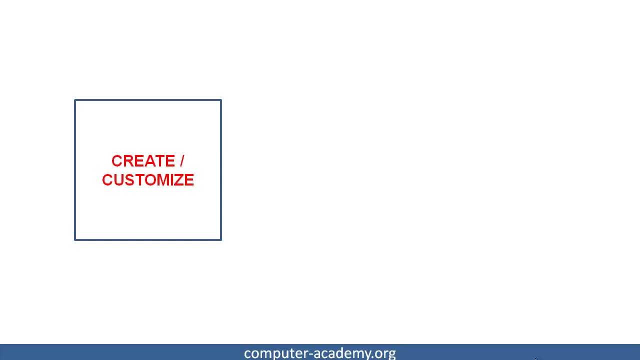 number of people. It also faces the highest number of challenges. So what do computer professionals actually do? We are now ready to take a quick peek into answering that question. They help create new applications or customize existing applications, and when they are ready. 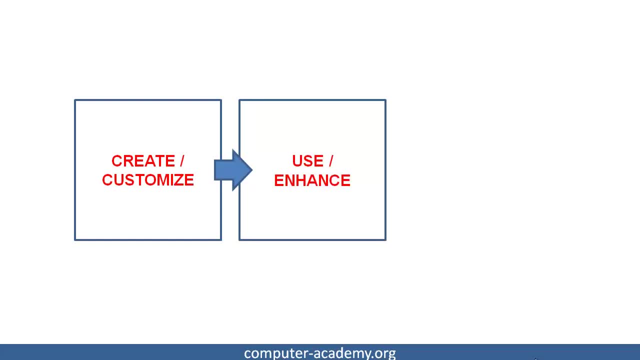 help users to use it. They enhance it to make it better and, after many months or years of using it, they help to replace or retire it When an application has been created. it costs the organization a lot of money. It costs the organization a lot of money. 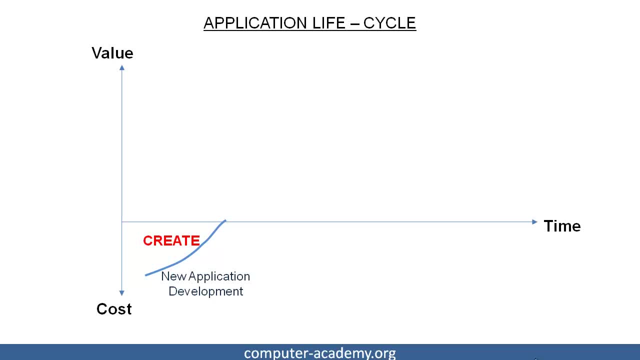 It costs the organization a lot of money When it goes into use. the organizations make money or save money by having users use it. Organizations continue to invest more money by making enhancements and changes to keep making it more and more useful to users, But as it gets older its value gradually decreases and at some point it costs the 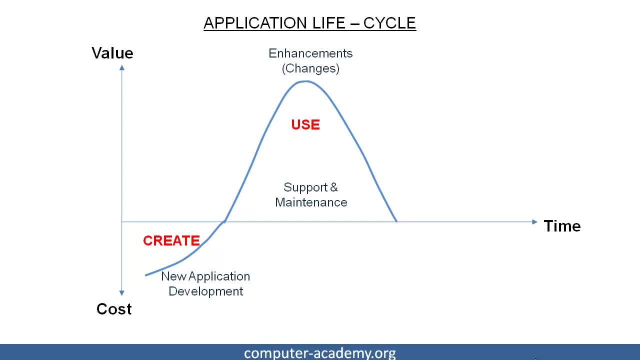 organizations more money to keep it going than the value it earns from it. At this point, the organization replaces or retires the application. Organizations continue to find ways to do more with scarce resources such as time, money and people. That means looking for ways to produce the same things quicker and cheaper. 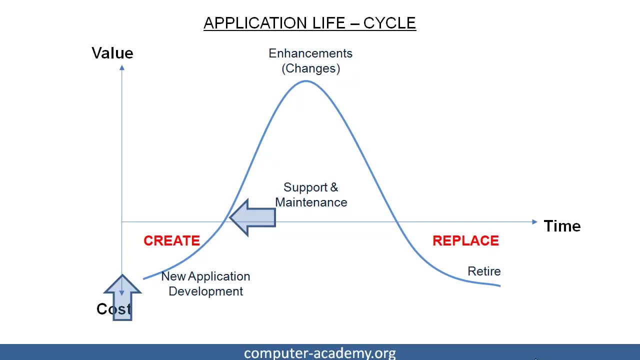 The same thing applies to creating and managing applications. Organizations are always trying to find ways to reduce the cost and time needed to create new applications. Increase the length of time that an application is in use before it needs to be replaced. Increase the value of the application so that users might use it for longer and use it more. 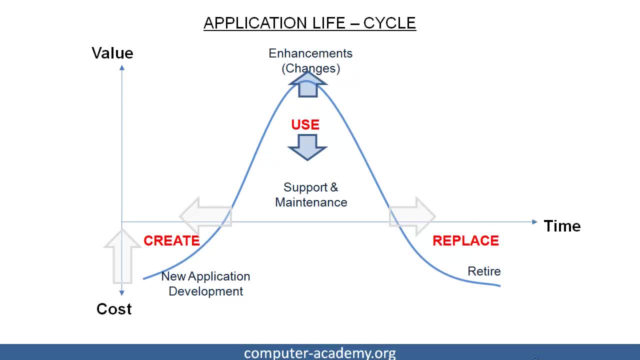 frequently, Applications need people and hardware infrastructure to keep it running. Organizations are looking to keep these support and maintenance costs as low as possible. When it comes time to replacing or retiring the application, organizations are looking to get rid of the cost. They need people and hardware infrastructure to keep it running as quickly and as cheaply. 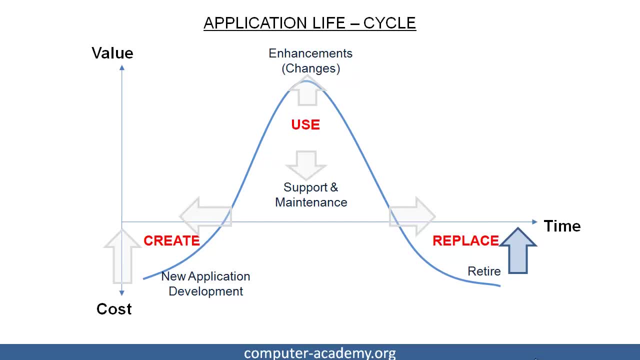 as possible. Software programming is only one aspect of the whole life, of managing an application from start to end. Most organizations often have more than one application. They typically have tens, hundreds and sometimes even thousands of such applications. To truly see what's going on, we need to step back and look at a wide range of topics. 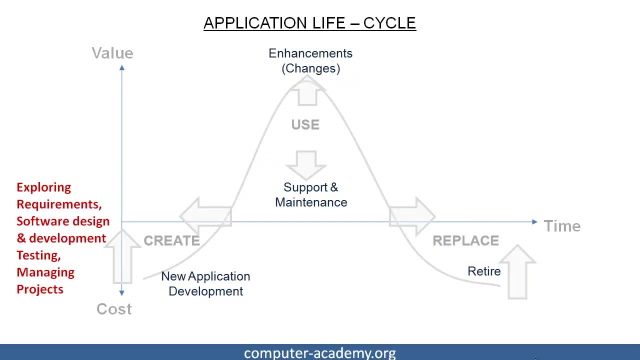 From the various ways to explore users' requirements, design software to reduce the time and cost of building testing applications, how to lead software and development teams and manage projects. we will look at ways to increase the value of applications already in use, how to decrease the support and maintenance costs, and what it takes to safely replace.